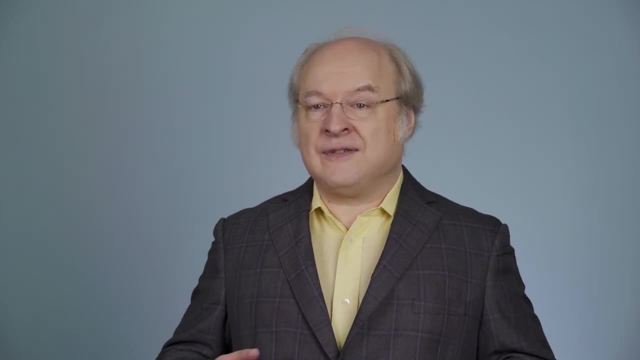 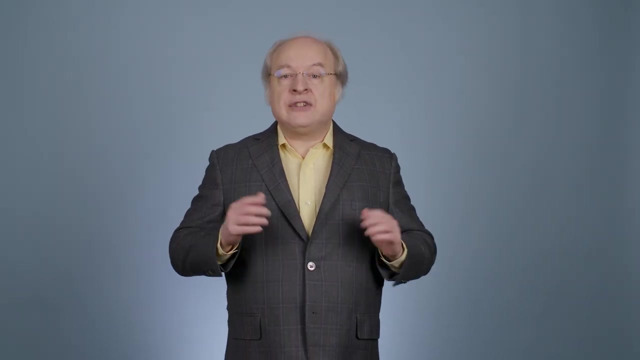 lot of user testing if you think about launching a product that violates any of the top ten usability heuristics. We have separate articles and videos for each of the ten heuristics, but just to give you an example if you want to learn more about usability heuristics. 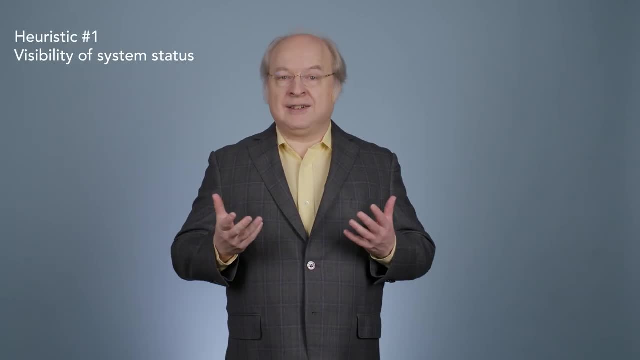 you should check out the video on the left. Heuristic number one is visibility of system status. This means users should always be able to tell what the computer is doing and what state it's in. They should not have to guess or remember things. The system should show them and give good feedback. 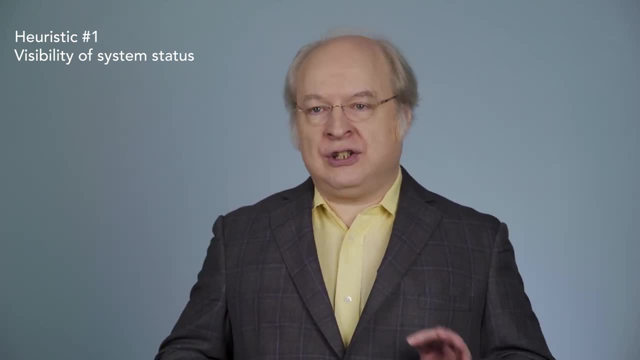 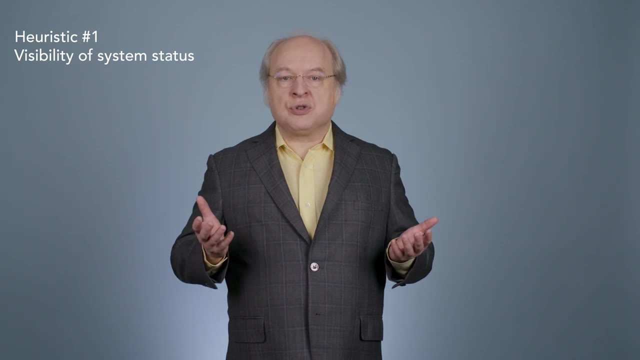 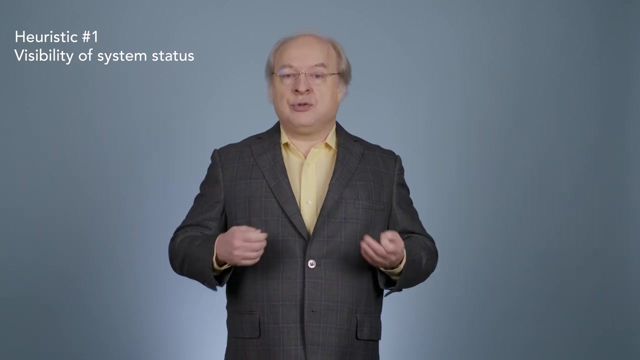 Now, that's a really general rule and, as with all ten heuristics, it applies across all types of computer technology. It doesn't matter whether it's a mainframe computer, a PC, a mobile phone or a smartwatch. Also, it doesn't matter whether you're designing. 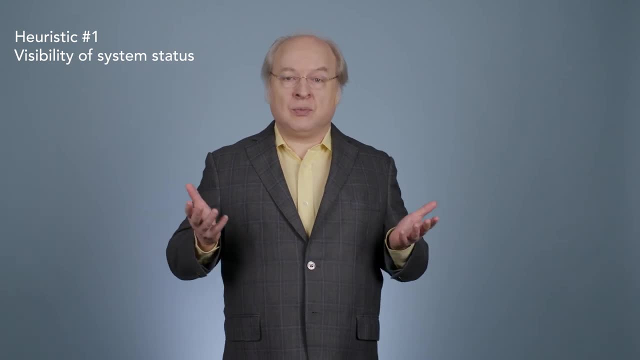 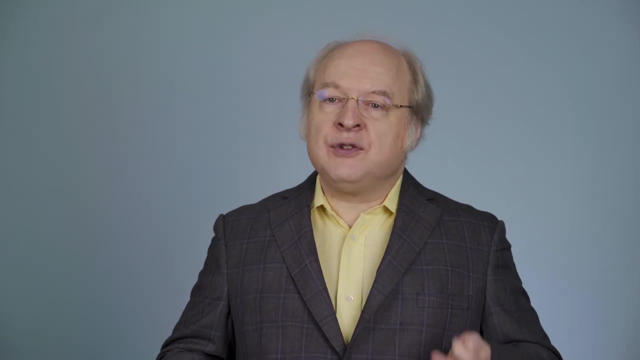 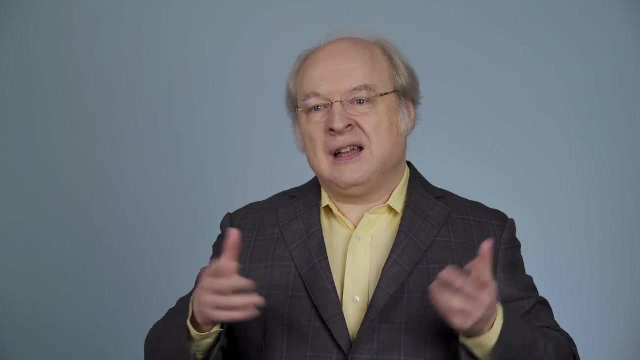 a video game, an enterprise application or a consumer website. In any case, you should aim for visibility of system status. Now, of course, if you're designing an auditory user interface, such as a voice assistant, we have to interpret the rule of visibility a bit differently. It's more a matter of the 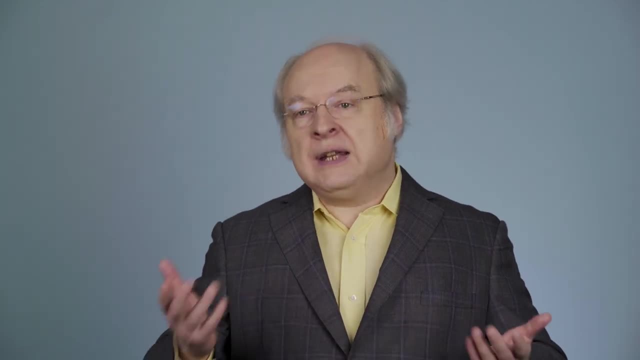 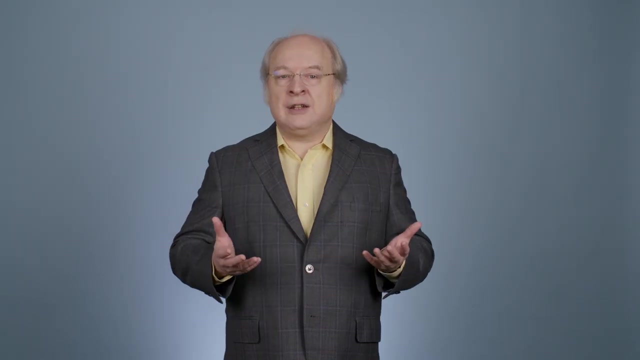 status being easily available and noticeable by the user, Even if the information is provided by, maybe, sound effects or spoken words. The top ten usability heuristics have remained the same for more than 25 years, exactly because they're so broad. They come from the basics of human behavior and the basics of what makes 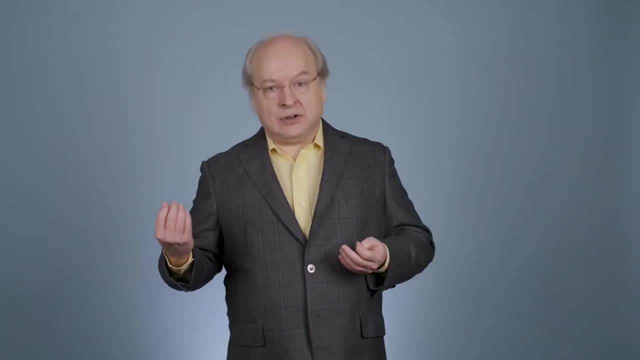 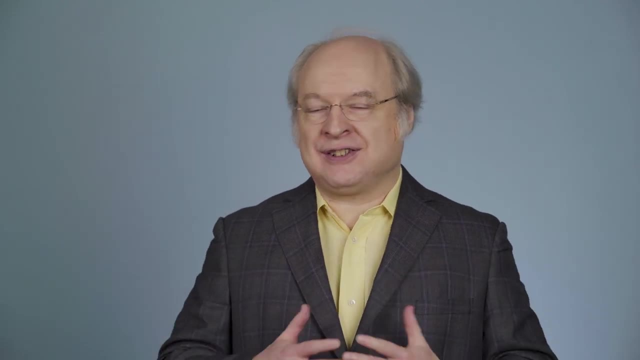 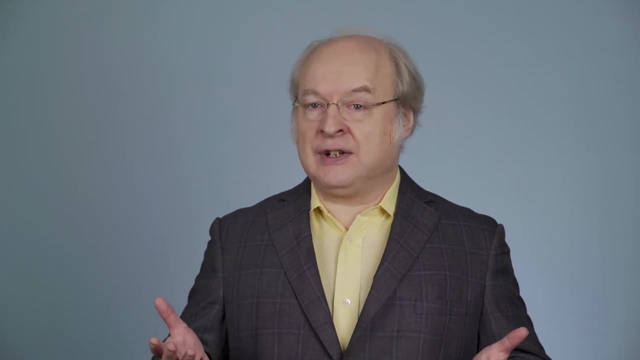 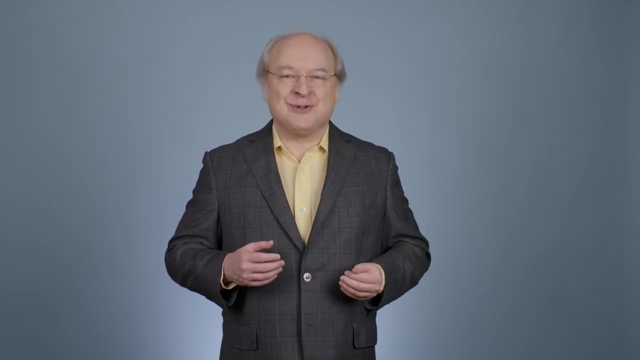 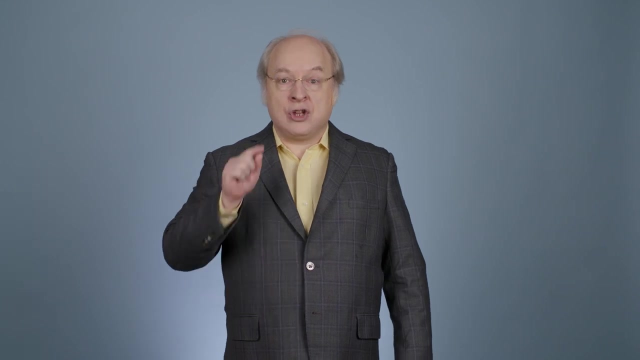 that they will also be relevant for future generations of user interfaces, decades from now. Because the heuristics are so durable, it's well worth the investment for you to spend the time to learn all ten of them and think about how they apply to the designs you are. 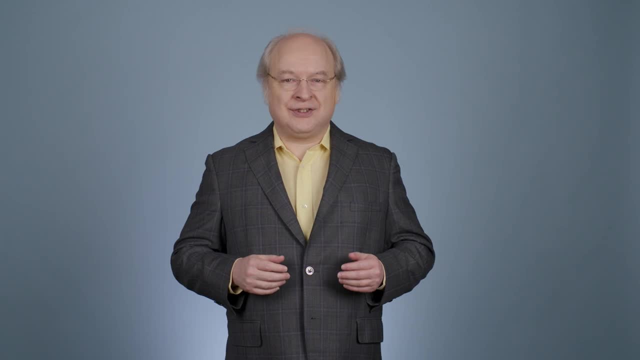 working on. See the list of all ten UX heuristics on the NN Group website, http//wwwnngroupcom.